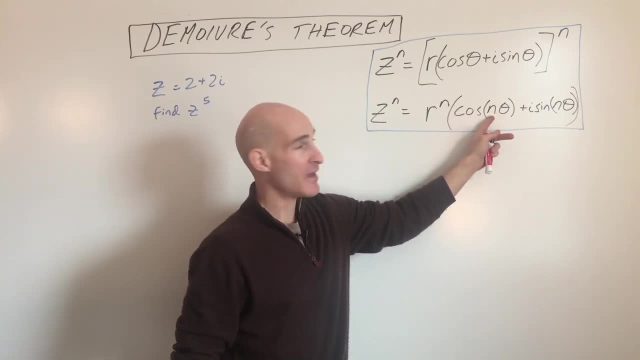 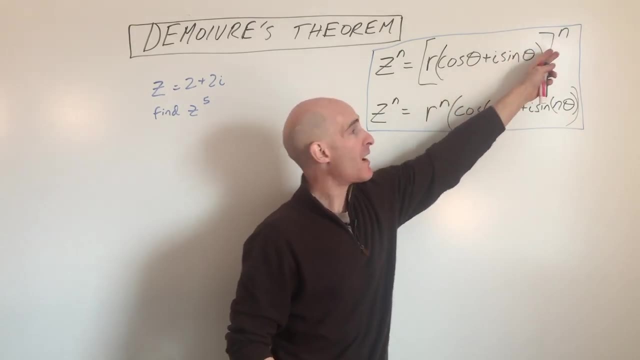 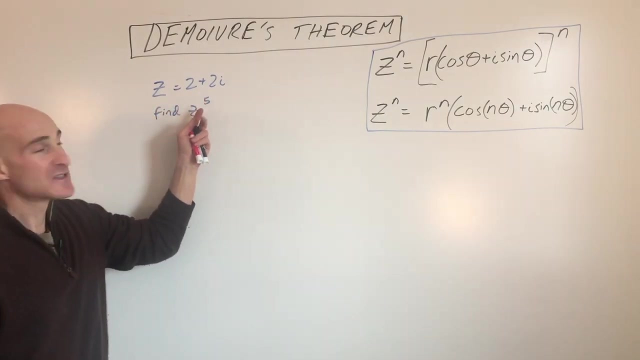 but you're going to multiply the angle by the nth power. okay, So this is how you take it: from a- you know just the trigonometric form- raise to a power, you just raise the r value to that power and you multiply the angle by the power. Let's look at an example. Say we want to find out. 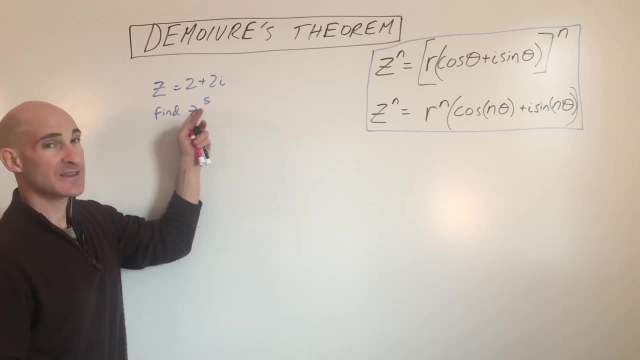 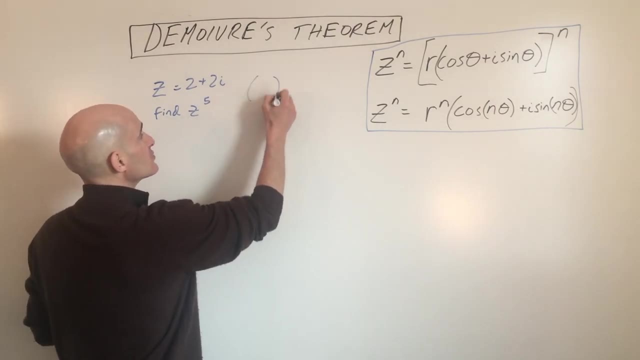 okay, if z equals 2 plus 2i. z's are a complex number. we want to find z to the fifth power. Now, if we wanted to do this a long way, we could take 2 plus 2i times 2 plus 2i. 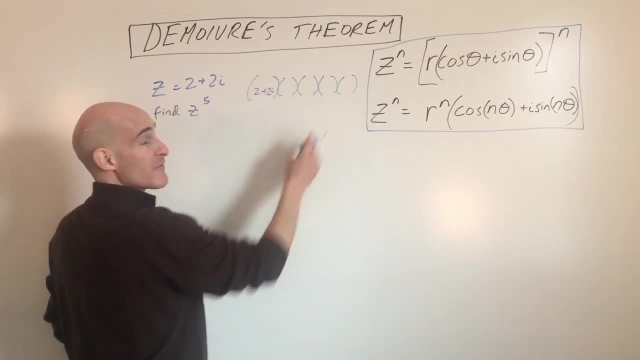 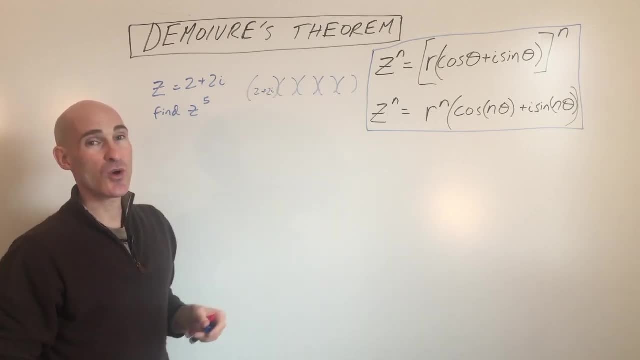 and you'd have to do the distributive property: simplify, distribute and so on. It would take a long time. So what we're going to do is we're going to use De Movert's theorem, we're going to convert this to the trigonometric form. I like to draw a diagram just to see what I'm working with. 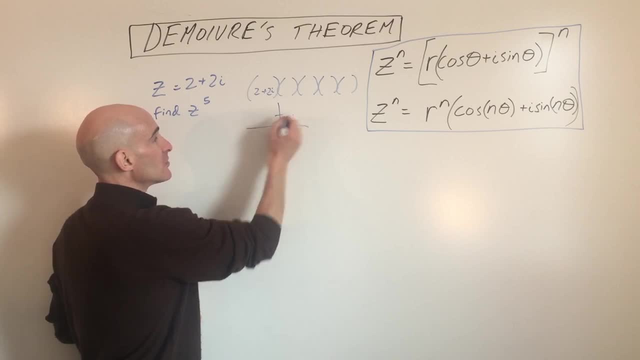 here, 2 plus 2i means you're going right to and up to. there's your point in the complex plane and there's the r value right there and there's the angle right there. So what we're going to do, 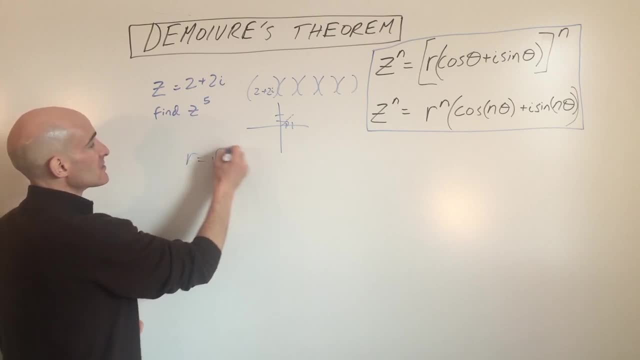 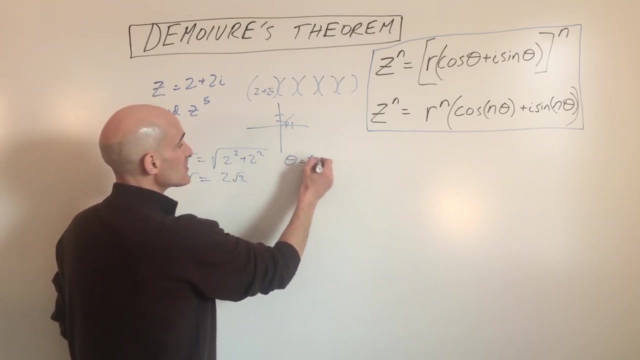 we're going to do. r equals the square root of a squared plus b squared, okay, which equals 4 plus 4, which is square root of 8, which is 2 root 2, so that's our r value. Theta equals the tangent inverse of b over a, which is 2 over 2, this is 1,. 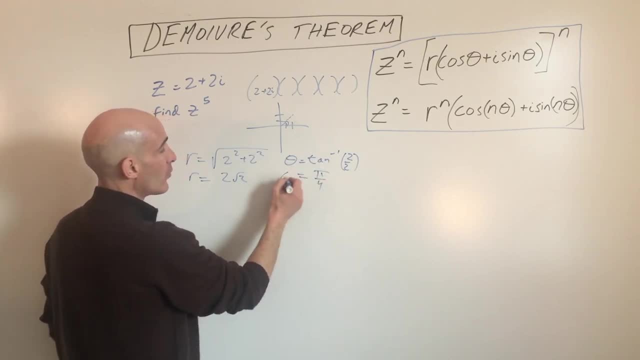 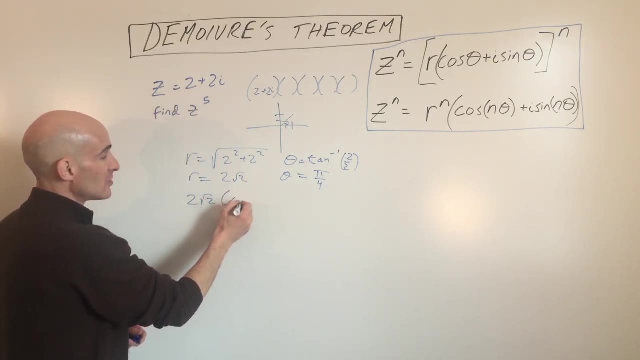 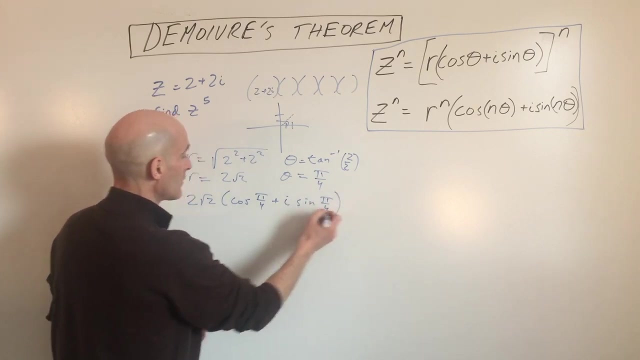 tangent equals 1 at 45, or pi over 4, and you can see this is pi over 4.. So if we write this in trigonometric form, what we have is 2 root, 2 cosine pi over 4, plus i sine pi over 4,. okay, so there's our complex number, the same number here. 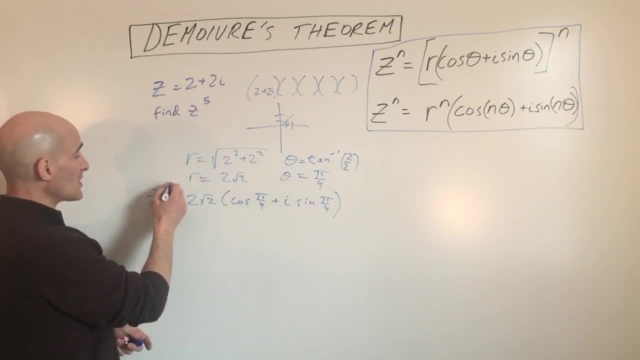 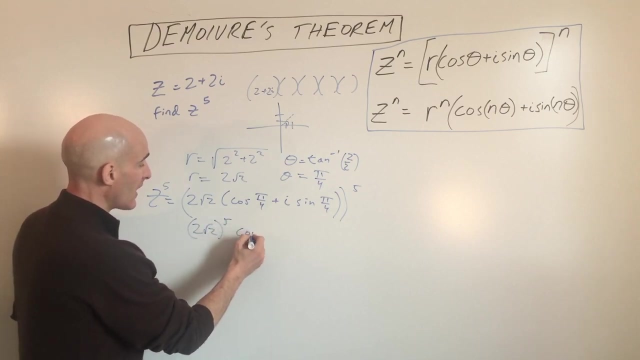 just in a different form, trigonometric form. Now, what we're going to do is we're going to raise both sides to the fifth power. We're going to use De Movert's theorem. we're going to raise the r value to the fifth power, so that's 2 root 2 to the fifth, and we're going to multiply the angle. 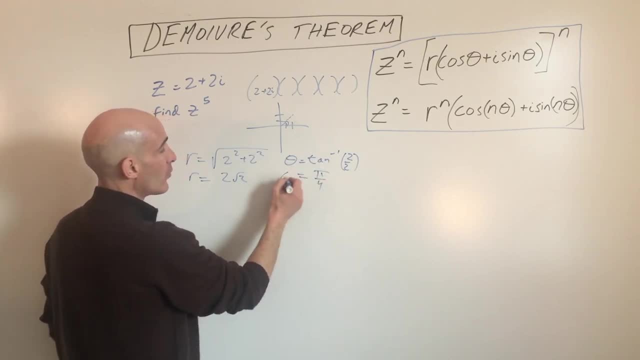 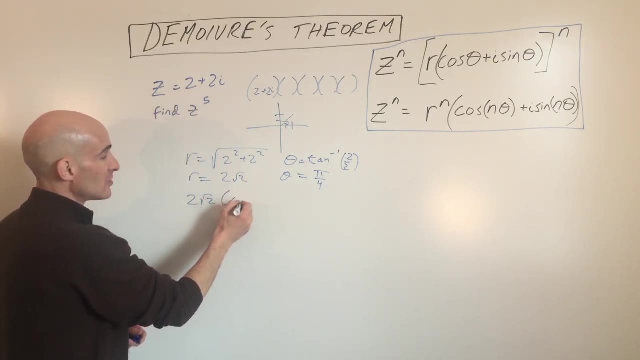 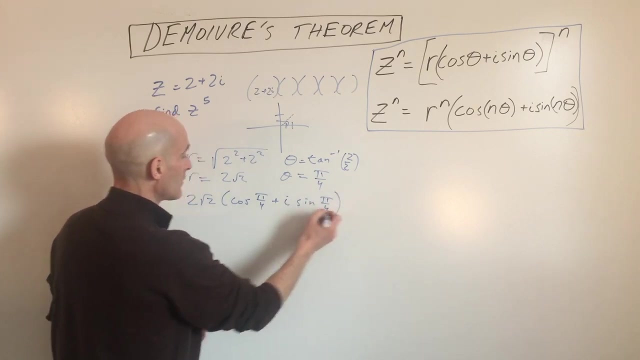 tangent equals 1 at 45, or pi over 4, and you can see this is pi over 4.. So if we write this in trigonometric form, what we have is 2 root, 2 cosine pi over 4, plus i sine pi over 4,. okay, so there's our complex number, the same number here. 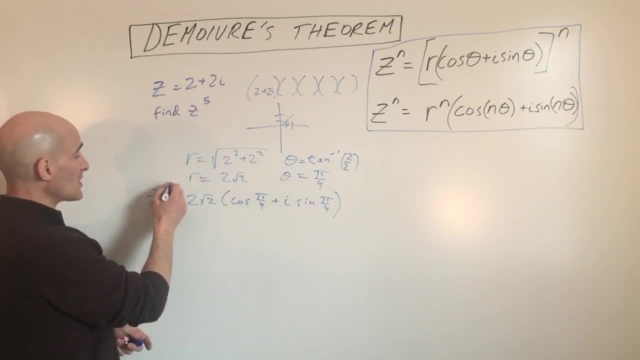 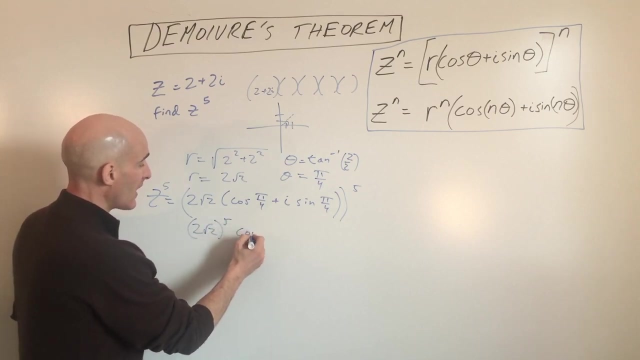 just in a different form, trigonometric form. Now, what we're going to do is we're going to raise both sides to the fifth power. We're going to use De Movert's theorem. we're going to raise the r value to the fifth power, so that's 2 root 2 to the fifth, and we're going to multiply the angle. 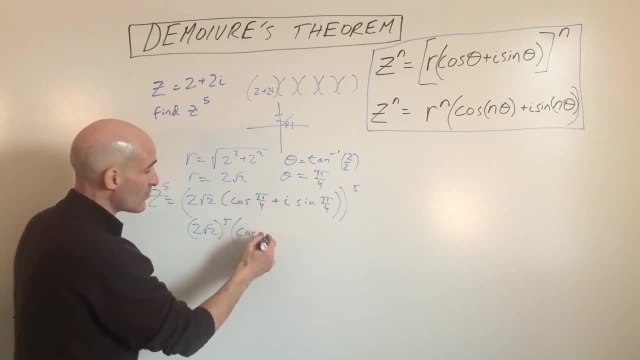 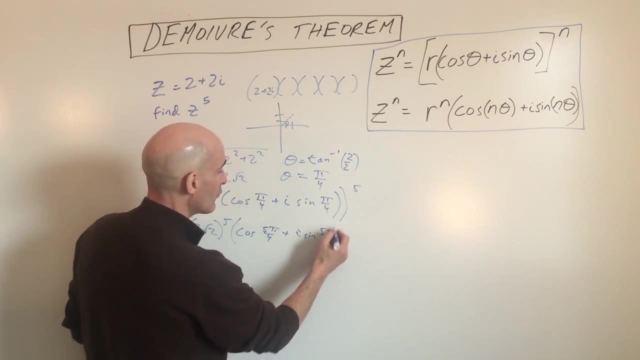 by 5.. So we're not raising it to the fifth power, we're just multiplying it by 5, so that's 5 pi over 4 plus i sine 5 pi over 4,. 2 root 2 to the fifth, 2 to the fifth is 32,. 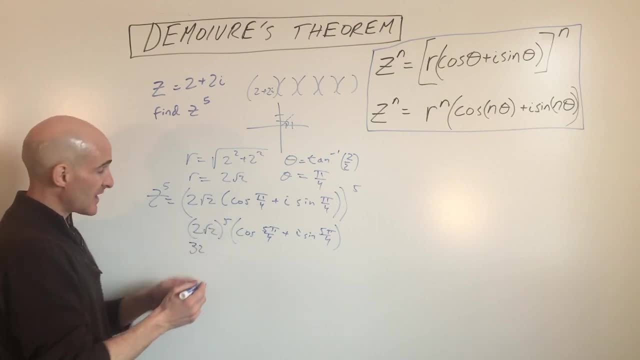 square root of 2 to the fifth is actually going to be 2 times 2 is going to be 4, times 2 is 8, times 2 is 16, times 2 is 32,. square root of 32 is 4 root 2,. 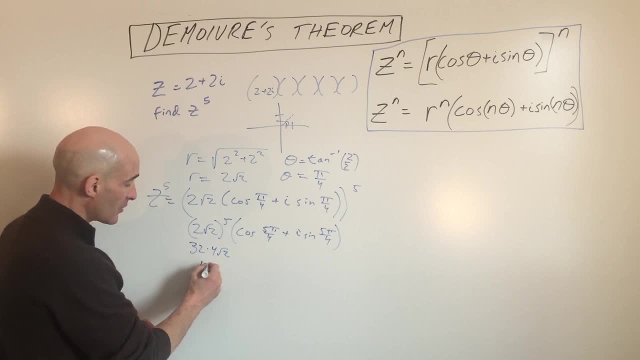 so that's times 4 root 2, so we get 128 square root of 2,. okay, and then cosine of 5 pi over 4 is actually going to give us negative root 2 over 2, and sine of 5 pi over 4 is negative. 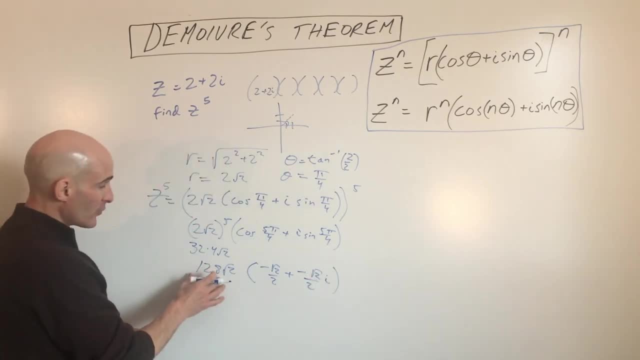 root 2 over 2 i. so if we distribute, we get 128 divided by 2 is 64, square root of 2 times square root of 2 is 128, times the negative, that's negative 128, same thing here. so that's going to be negative 128 i. so this is a lot faster way than having 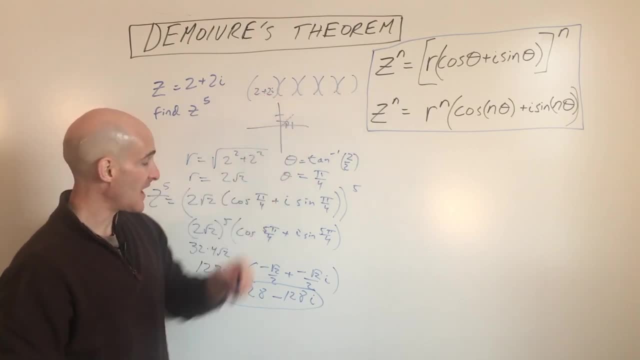 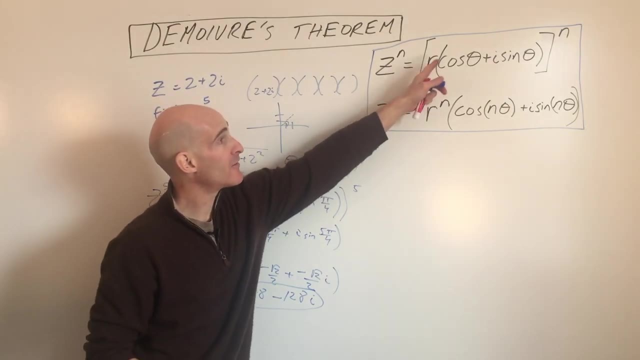 to foil out this binomial 2 plus 2, i, 5 times. what you can do is just translate it into the trigonometric form and use De Movert's theorem by taking the r value to whatever power you're working with and then multiplying that power's value times the angle. and then, if you want, 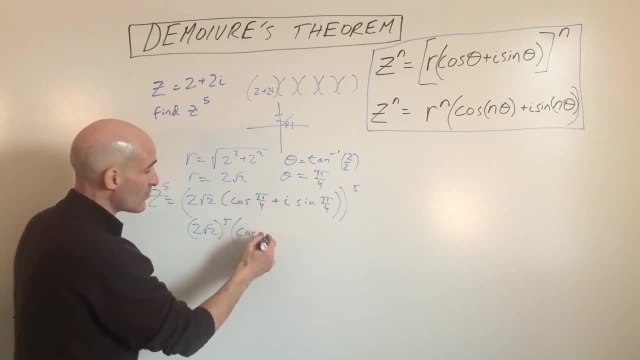 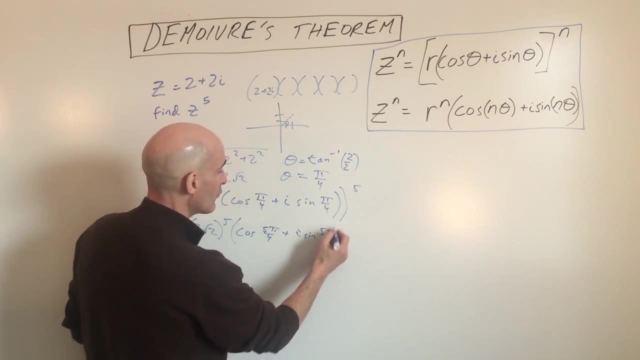 by 5.. So we're not raising it to the fifth power, we're just multiplying it by 5, so that's 5 pi over 4 plus i sine 5 pi over 4,. 2 root 2 to the fifth, 2 to the fifth is 32,. 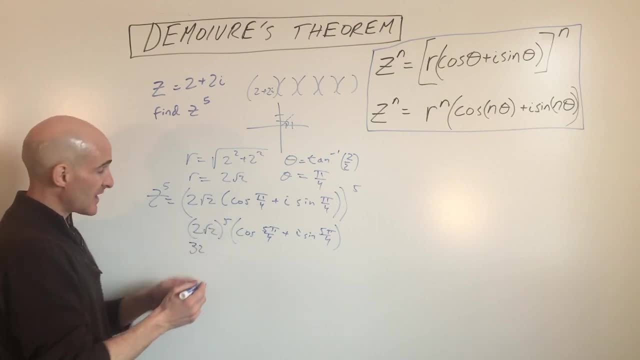 square root of 2 to the fifth is actually going to be 2 times 2 is going to be 4, times 2 is 8, times 2 is 16, times 2 is 32,. square root of 32 is 4 root 2,. 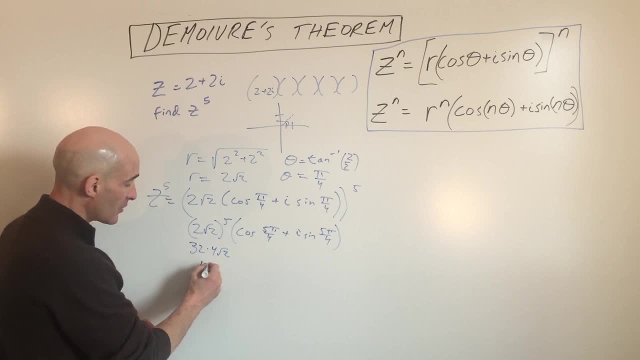 so that's times 4 root 2, so we get 128 square root of 2,. okay, and then cosine of 5 pi over 4 is actually going to give us negative root 2 over 2, and sine of 5 pi over 4 is negative. 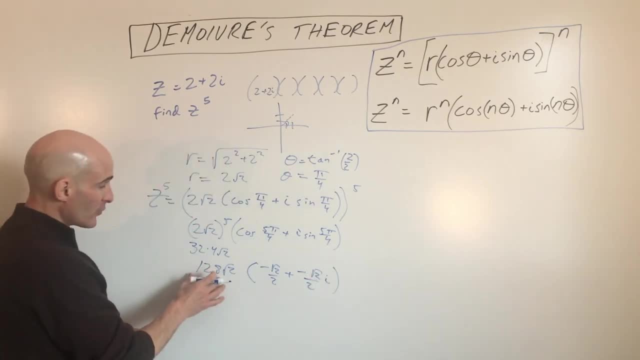 root 2 over 2 i. so if we distribute, we get 128 divided by 2 is 64, square root of 2 times square root of 2 is 128, times the negative, that's negative 128, same thing here. so that's going to be negative 128 i. so this is a lot faster way than having 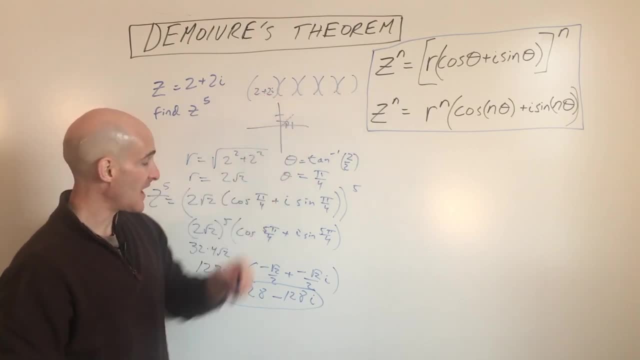 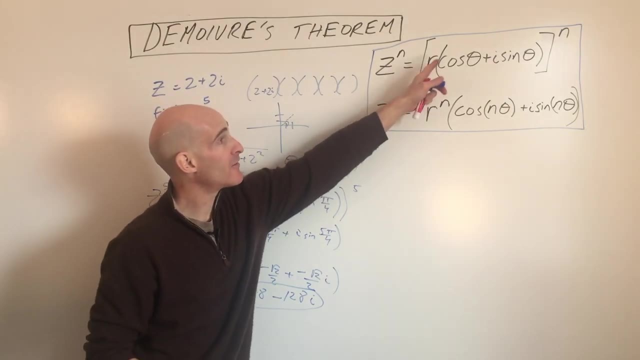 to foil out this binomial 2 plus 2, i, 5 times. what you can do is just translate it into the trigonometric form and use De Movert's theorem by taking the r value to whatever power you're working with and then multiplying that power's value times the angle. and then, if you want, 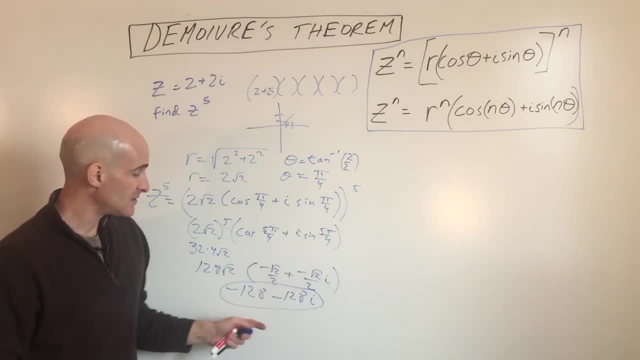 you can then distribute: okay, this r value back in to change it back into the standard form of a complex number, the a plus b i form. so this has been how to work with De Movert's theorem. I'll see you in the next video.